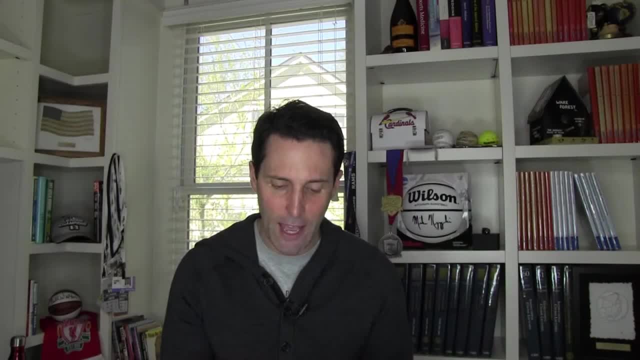 you ask her, she's ready to get back out on the floor and on the field. As her parent, I want her to encourage her to do all that she wants to do, but provide the safety structure that she's not able to understand yet. I personally see the benefits of the cross. 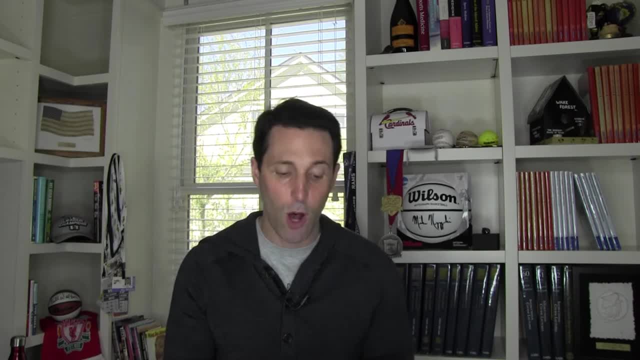 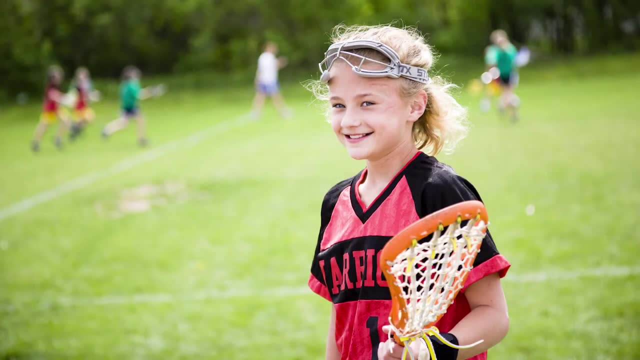 conditioning that gymnastics provides, but our lacrosse coach, who also happens to be her dad, is encouraging her to only do one sport at a time. All right, so there's two things to talk about here. One is gymnastics: more injury prone. than lacrosse. You know it would depend on the different studies you look at and it's hard because you're comparing apples to oranges, but I would argue they're not really more or one's not more dangerous than the other, It's just a different set of injuries. Gymnastics. 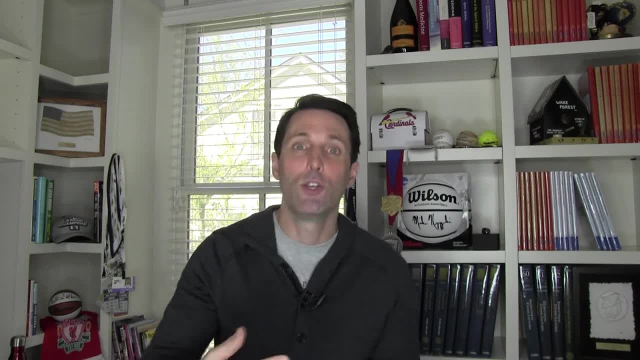 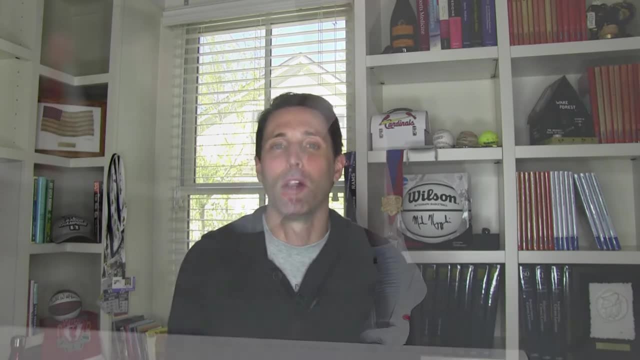 is unique in that it's an upper body weight bearing sport, so you can have upper and lower body injuries. but I'm fine with it if athletes really want to do it. I wouldn't pull them out just for an injury risk, necessarily. I would just do it safely. Spotters and proper. 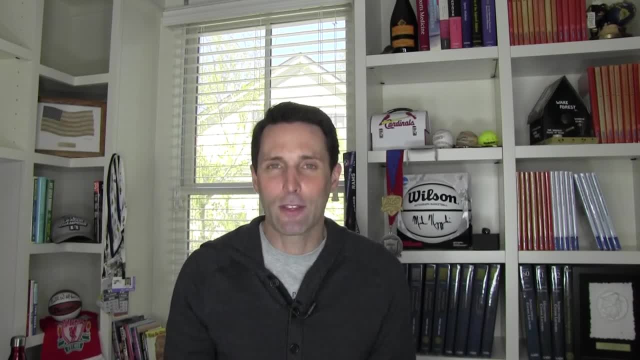 techniques and all of that kind of good stuff. Here's what I think the more important point is. no, I am strongly in favor of playing multiple sports. I think where people get into trouble is doing one sport all year round without a break. Yes, coaches love only playing one sport because they want to win, and so 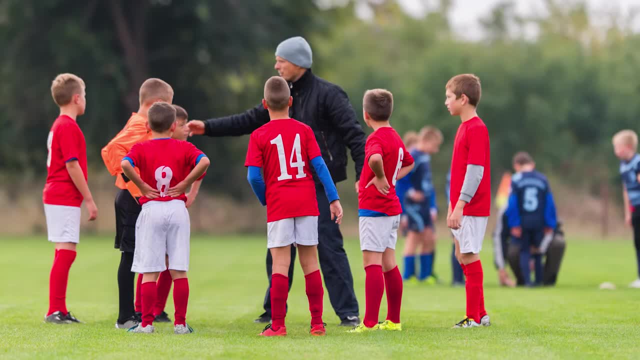 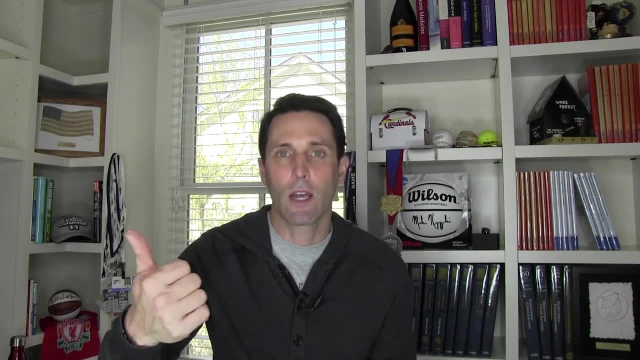 they think that if you play one sport year round you're going to get better at that one particular sport. but there's tons of evidence that you're actually more likely to play in college and make the pros at an elite level playing multiple sports. It lowers. 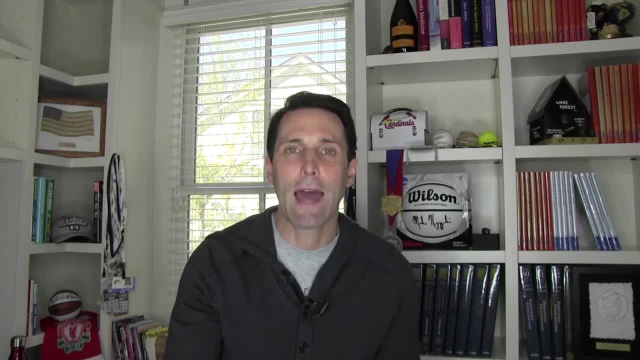 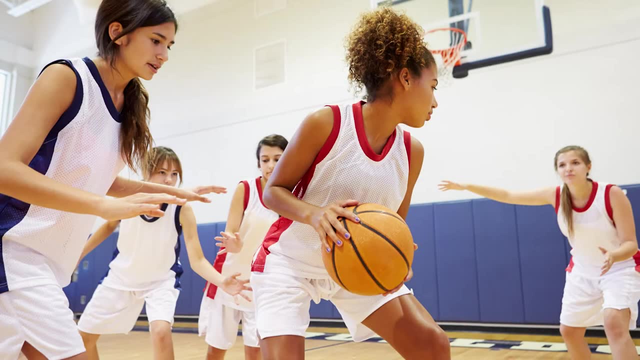 the stress to different parts of the body. so if you're a running athlete six months a year but then you do a throwing sport or a shooting sport like basketball, it moves the stress to the upper body for a period of time, giving those body parts time to rest. 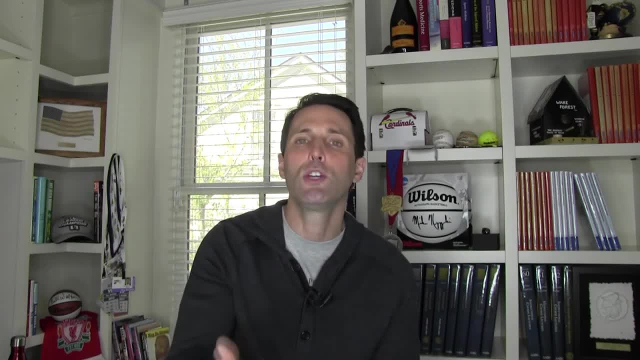 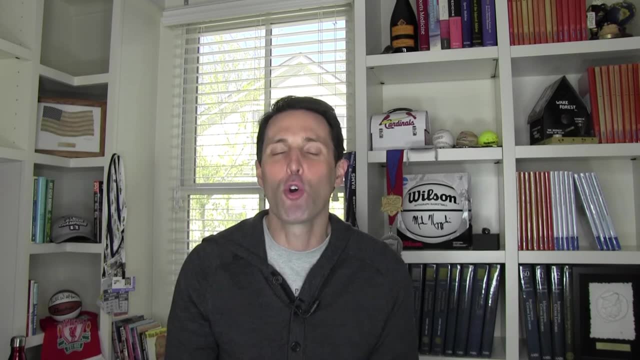 but it also teaches movement patterns that are different and better coordination and a lot of skills that you won't get if you only play the one sport year round. I think there's no question. I'm strongly in favor of letting a kid play multiple sports.